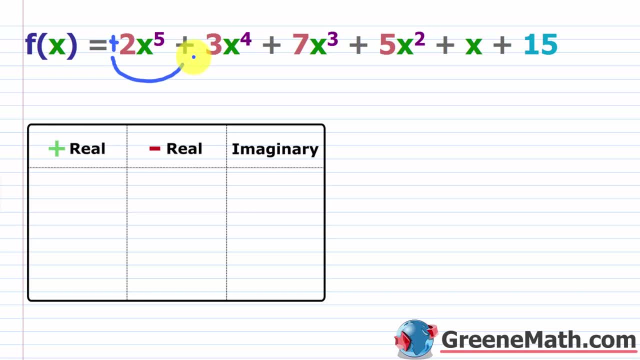 and I'm going to say from here to here: there's no sign change right. Positive to positive signs: the same Same, same, same Right. So there's no sign changes at all. right, It doesn't change. So that means there's zero sign. 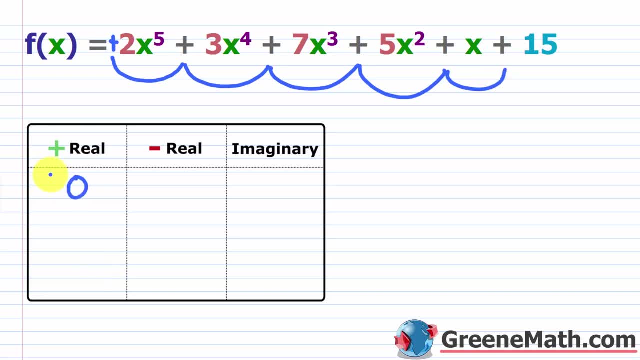 changes. So we're going to put a zero here, And that means there's zero possible positive real solutions. Okay, So that's what that means. Now, if it's not zero, okay, then what you want to do is you want to say you can have that number or you could subtract away two from that number. 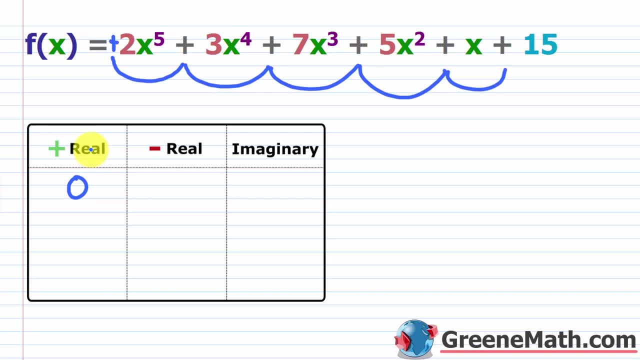 until you get to zero or you can't subtract away two anymore. Okay, So I'm going to give you an example in a moment of what I'm talking about there, But for right now there's zero sign changes, So there's zero possible positive, real solutions. Okay Now. 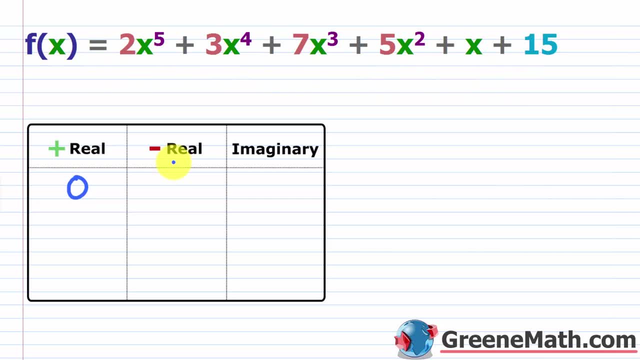 let's talk about negative. So for negative real solutions, what you're going to do is plug in a negative x everywhere there's an x in your function. Now I'm going to give you a little shortcut for this. Don't go through and actually start plugging things in, because the sign is only 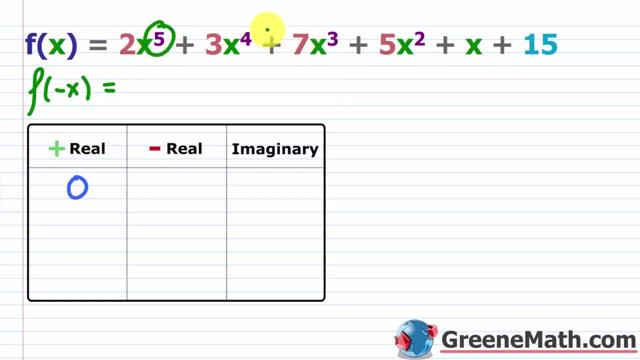 going to change Okay, Exponent, right. So here, here, and then this is the first power. So here, if I think about it, I'm really just plugging in negative one times x. So just think about the negative one part. 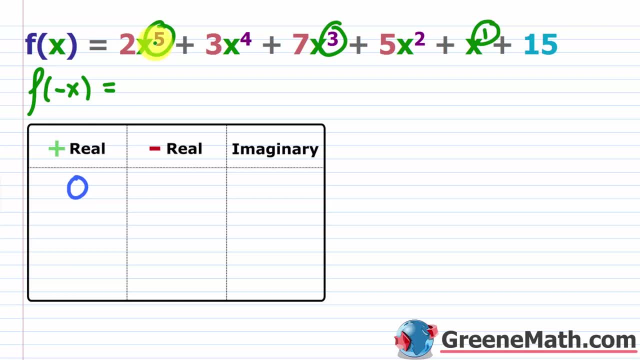 negative one raised to an odd power is going to give you back negative one. So it's going to change your sign. Okay, But if I had negative one raised to an even power, like negative one raised to the fourth power, it becomes one right. So no sign change. So I'm going to go through and 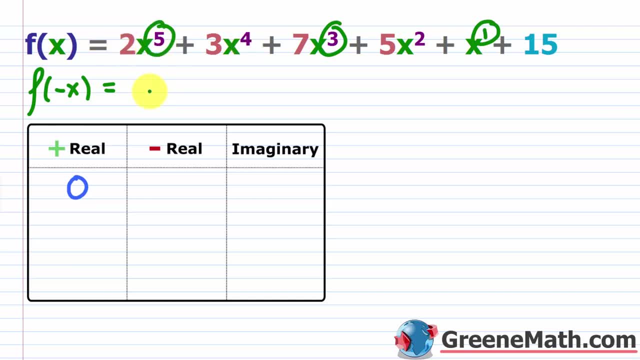 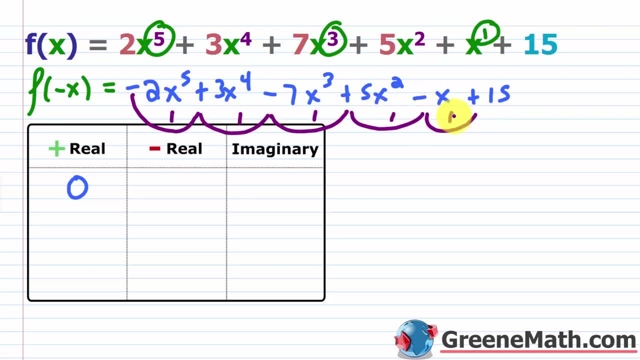 on them. So you got one, two, three, four, five. So we're going to put a five here for the possible negative real solutions. Now here's where this gets a little bit tricky, Okay, When you think about the imaginary solutions that are possible, where the non-real, complex solutions, remember. 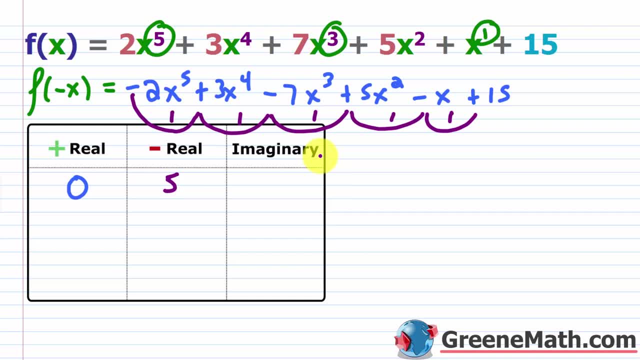 they come in conjugate pairs. So right now, if this was the scenario, you would have zero, because this is a fifth degree polynomial right. So you're going to have five solutions. Again, some of those could be repeats, but you're going to have five solutions, or five roots or five zeros. 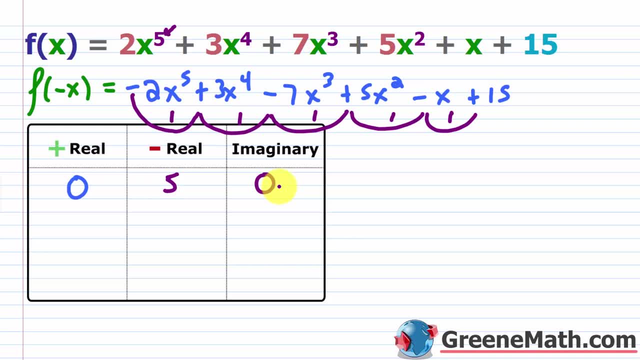 however, you want to say that Now there's other scenarios that could be possible. Again, when I talk about this, you're going to decrease this by two, whatever these numbers are, because, again, the complex solutions are the non-real complex solutions, The imaginary solutions are going to. 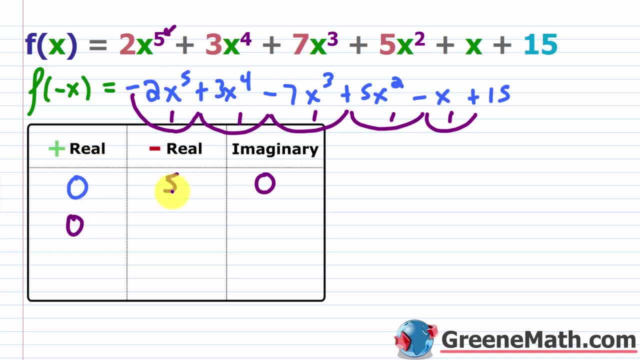 come in conjugate pairs, So I'm always going to have zero here, but this could be reduced by two. So I'd put three here, and now I'd put two here, because again, if I have one solution there, I've got to. 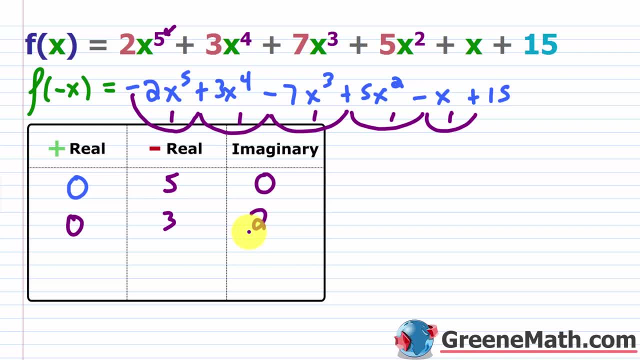 have two, It can only be zero. two, four, six, eight. It's got to be some even number. Now, if I decrease it again, this would still be zero, This would be one, And now this would be four. 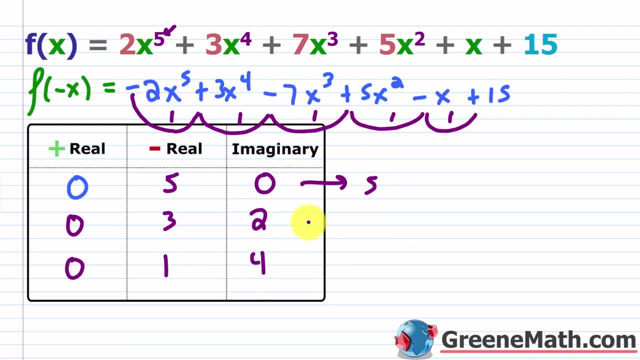 Okay, So notice how the total in the row is always five, right, The total is always five. So that's what you're looking for. So I started with five, I went down to three, Then I went down to one, Started with zero, went up to two, went up to four. Okay, 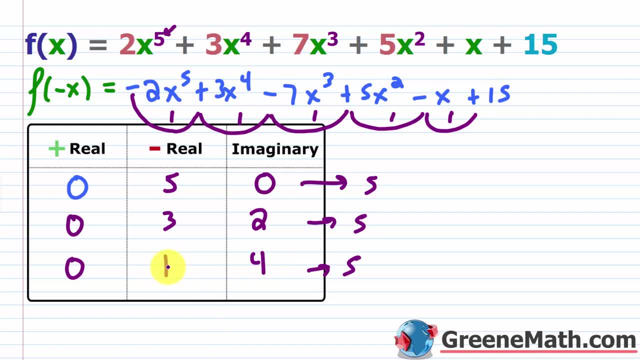 Now notice how I can't decrease this guy by two again, because that would tell me that I have negative one, negative real solutions. That's nonsense, right? That's not possible. So you need to keep going and reducing by two until you hit zero or something. that's not possible. 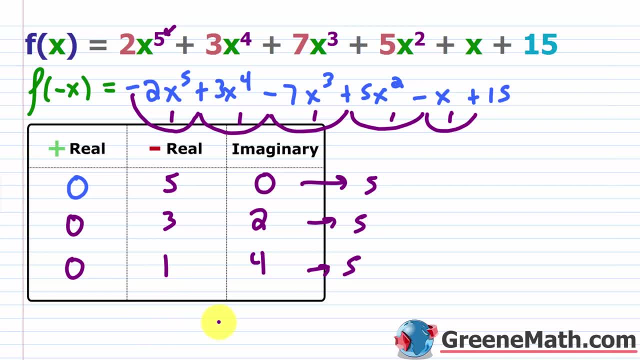 like in this case, right here. Okay, So for this example, we have one scenario where you have zero positive real solutions, five negative real solutions and zero imaginary solutions. Or you could have zero positive real solutions, three negative real solutions and two imaginary. 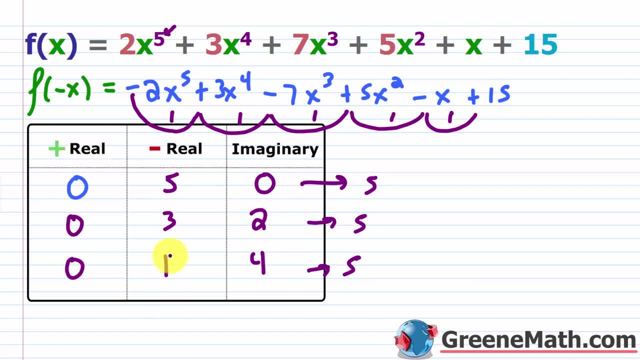 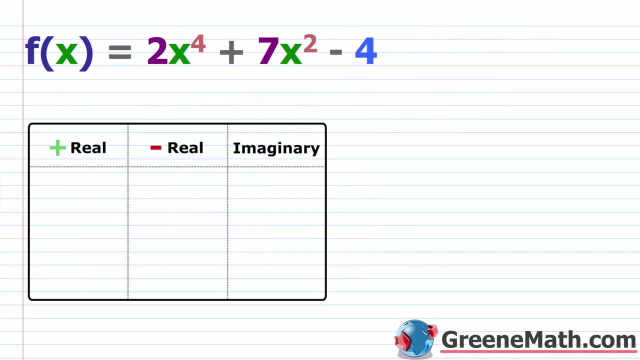 And then, lastly, you could have zero positive real solutions, one negative real solution and then four imaginary solutions. Let's take a look at another example. Once you do these a few times, it's very, very easy. So again, if I want to find the possible number of positive real, 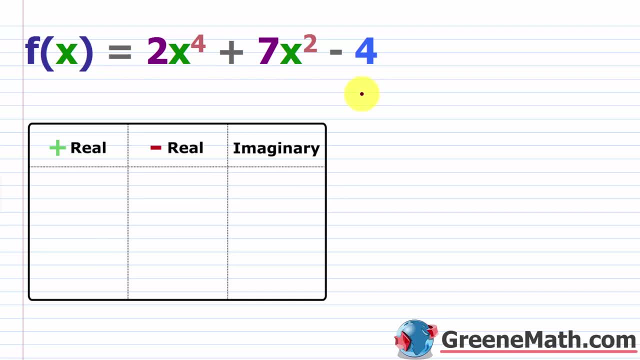 solutions. I just look at f of x. I make sure that again all my coefficients are real, and then I have a non-negative real solution. And then I have a non-negative real solution, non-zero constant term, which I have. You'll notice, here you're missing x to the third power. 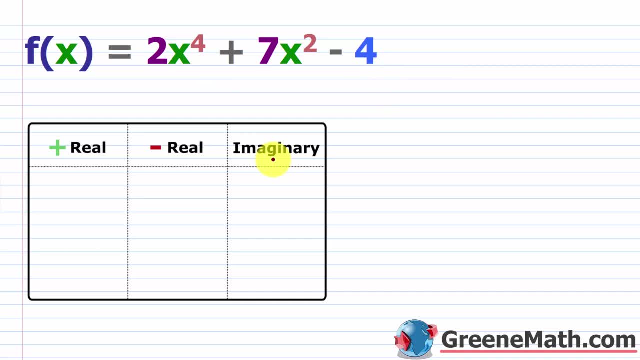 and x to the first power. That's okay, You don't have to worry about that, Just as long as you have this guy right here, your non-zero constant term, All right, So it's in standard form. So I'm just. 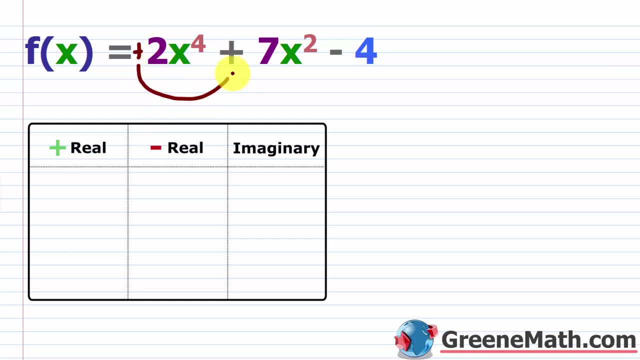 going to count my sign changes, So I go from plus to plus no change. plus to minus one change. So that tells me this could be one right here. Okay, Now this is a fourth degree polynomial, so I know there's more stuff coming, Okay. 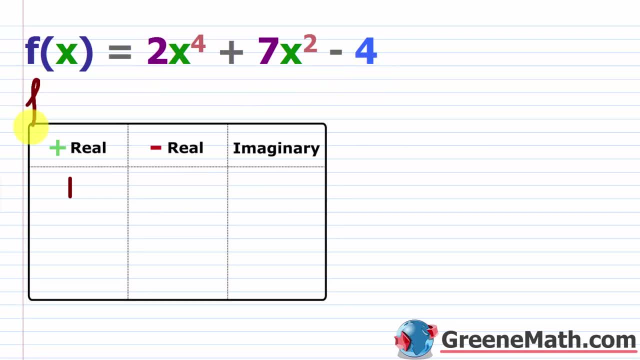 So I'm going to erase this. and let's think about f of negative x. Would anything change? No, because this is even, and this is even. So a negative one to the fourth power, or a negative one squared, okay, would give me positive one- no sign change. So this is two x to the fourth. 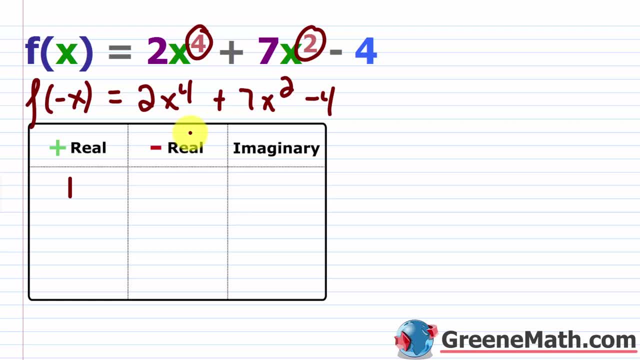 power plus seven, x squared minus four, So it's going to be one sign change again. You go from positive to positive, no change. positive to negative- one change. So really, what we find here is that there's only one positive. So we're going to go from positive to positive, no change. 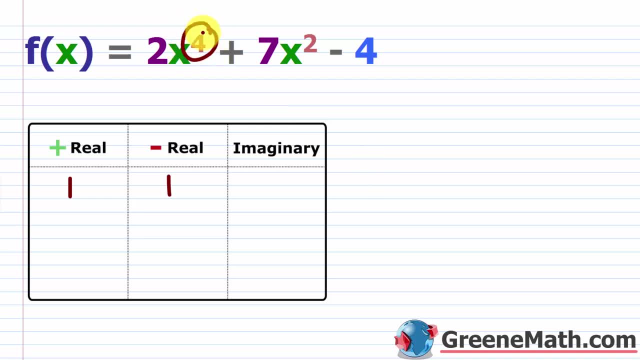 possibility because again, this is a fourth degree polynomial. This row here has to add up to four, So this has to be two right. Again, these come in conjugate pairs. So the only possibility is that you have one positive real solution, one negative real solution and two imaginary. 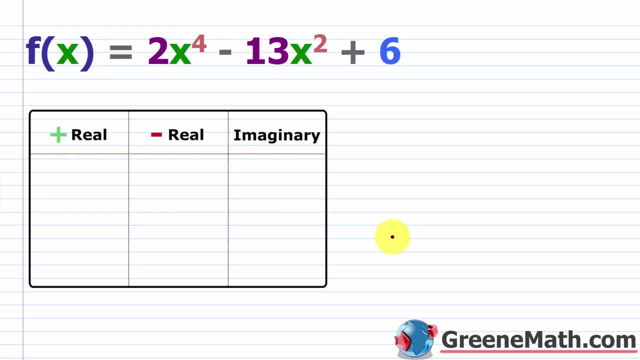 solutions. All right, Let's look at another one. So we have f of x equals two x to the fourth power minus 13, x squared plus six. So again I have a non-zero constant term, and then I have real coefficients. So I know I can use this. So again, just count the sign changes to get the possible. 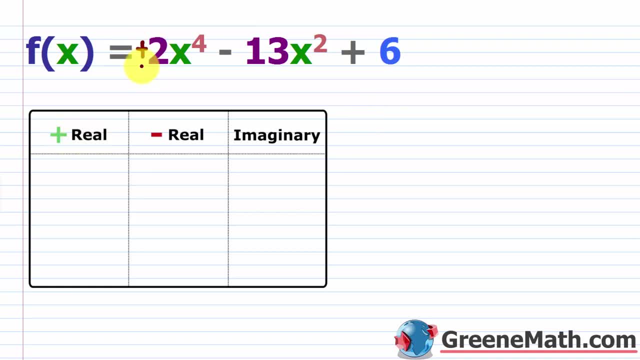 positive, real solutions. So this is plus. So going from here to here, that's one. Going from here to here, that's two. So I'm going to put a two there, And again I know I can decrease that by two. and 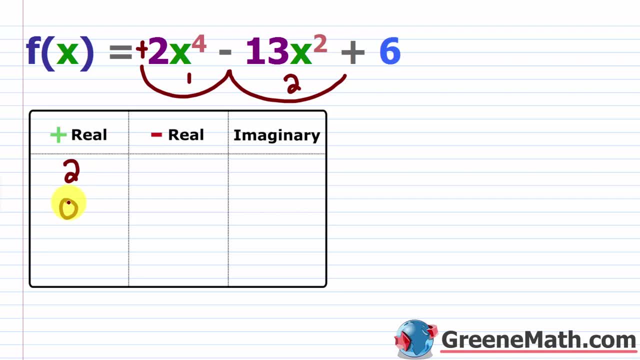 go to zero. So I can either have two positive real solutions or zero positive real solutions For the negative real solutions. remember, if you plugged in a negative x there, if I plugged in a negative x there, nothing would change, because this is even and this is even, So you'd have two sign changes again. 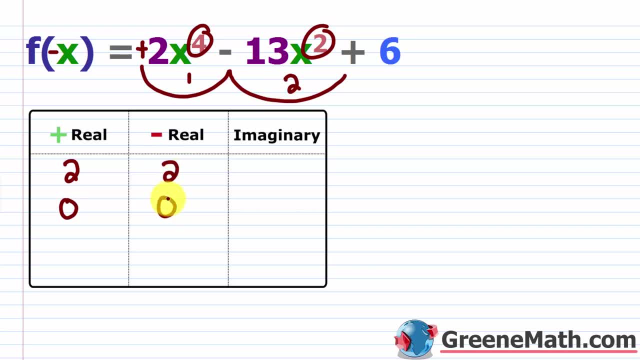 So let's go ahead and put two here and zero here, But you have another two scenarios that you have to consider. So you could have two positive real and two negative real And of course, because it's a fourth degree polynomial, you'd have zero imaginary. You could have zero positive. 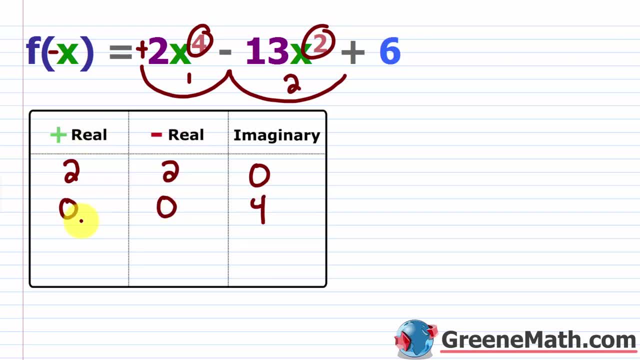 real, zero, negative real. and then you'd have four- imaginary Again, the row has to always sum to four. Then the other scenario would be: you could have two and zero, and this would be two. So two positive real, zero, negative real. 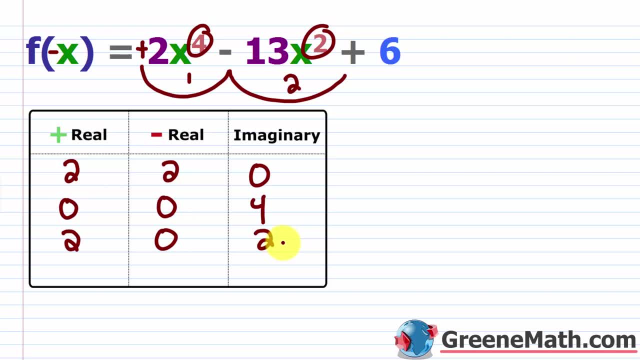 and two imaginary, And then the final scenario would be that you have zero positive real, two negative real and two imaginary. So again, when you go through the different possibilities, you want to think about the imaginary as being what's left over. So in this case, 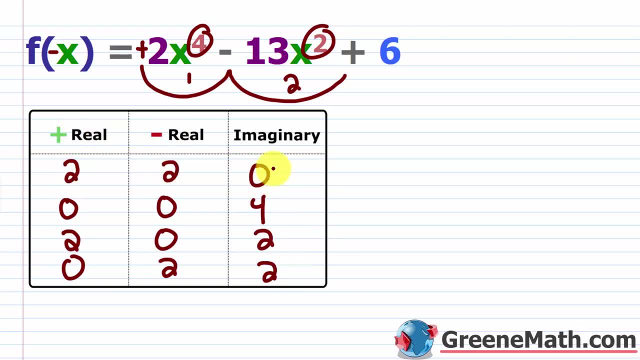 you have two positive real, two negative real, So there's nothing left over because you're going to have four solutions Again, this is a fourth degree polynomial, okay, So this guy: zero, zero, and then you get four right, Because there's nothing here. It's got to sum to four: Two, zero, and then this has to be. 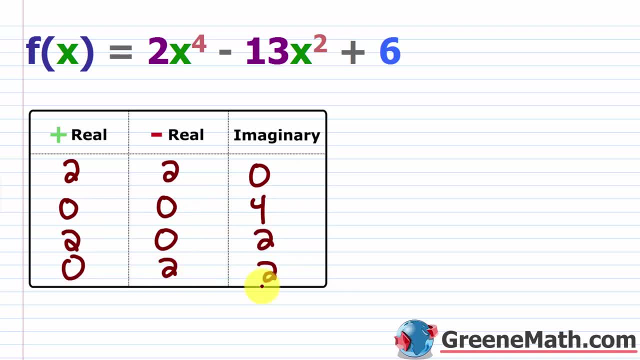 two, Two plus two is four, Zero two. and then again this is two, because two plus two is four. All right, Let's just look at one final example. So we have f of x equals 6x to the fifth power. 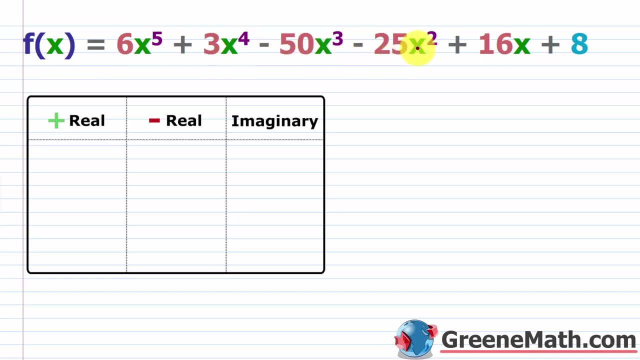 plus 3x to the fourth power, minus 50x cubed, minus 25x squared, plus 16x plus eight, Again I've got my non-zero constant term. All my coefficients are real numbers, So I'm good to go. So how many sign changes do I have? So no sign change. Then I've got one. 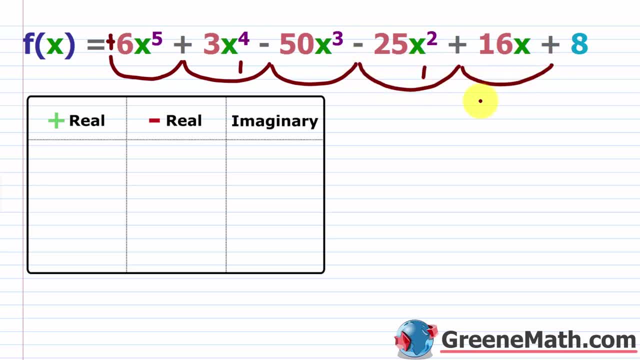 No sign change. I've got another one and no sign change. So this is going to be two. So let's put two here, And then we know it's also possible to have zero. Now, if I change this to a negative,